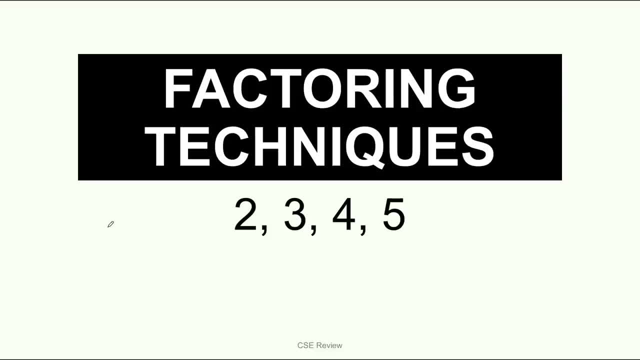 I'll see you in a bit, Alright, so today we're going to talk about factoring techniques: numbers 1, 2,, 3,, 4 and 5.. The other numbers- 6,, 7,, 8 and onwards- they're going to be discussed in the next. 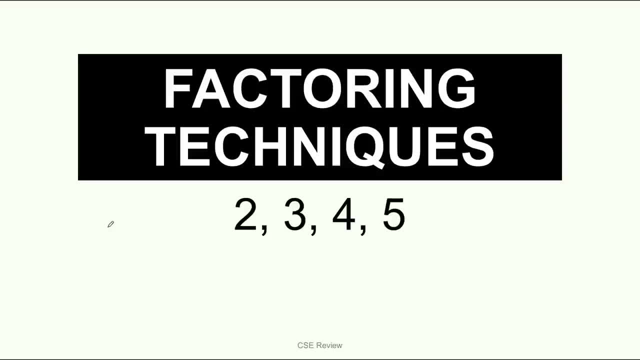 in the next video. The reason is because if you're not familiar with this technique and these four numbers at the beginning, it's going to be harder for you to deal with the bigger numbers. So our goal now is for you to master these four so that when it comes to bigger numbers, you'll be ready. 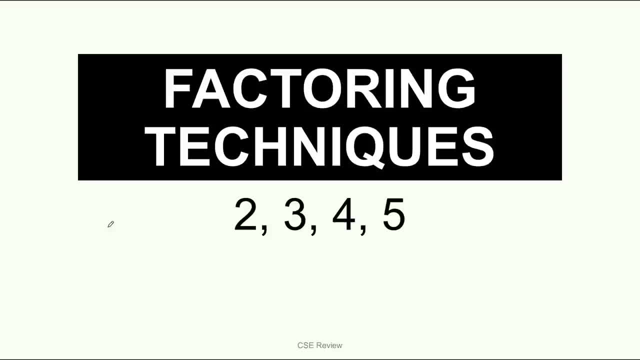 Alright, now I'll explain to you the rules for each number, and if you find it hard to figure out how to do it, you can watch it again and again until you understand it. Alright, and again at the end of the video we're going to have a free quick quiz, so make sure that you watch until the end. 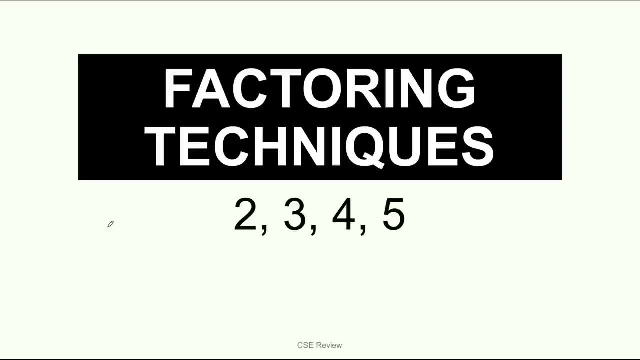 so you can access it, because it's best for you to practice on your spare time. A lot of my students would tell me that, coach, when I hear your voice or when you're in front of us teaching us live, it's easy to understand the concept. it's also easy to answer. but why is it that when I'm the only one? 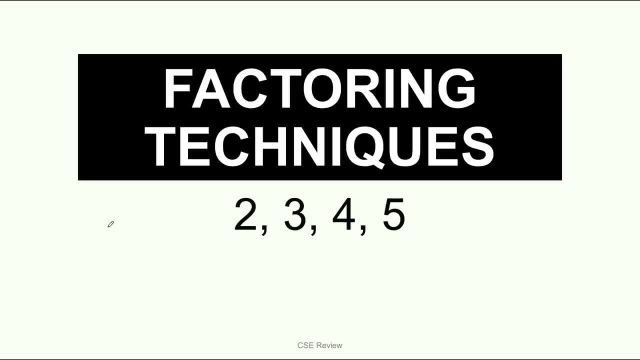 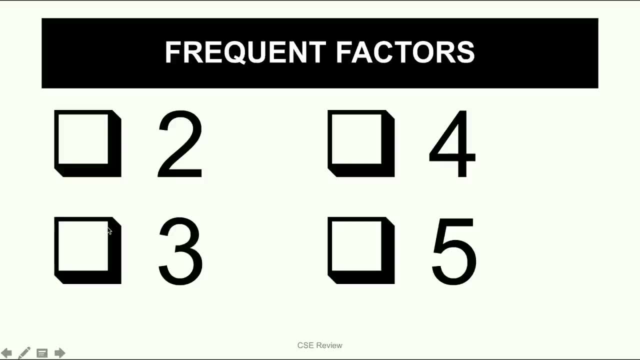 who's having a hard time Now, the key there really is personal practice, So you're going to have to set aside time to practice. Alright, now let's talk about these frequent factors. We're going to talk about two, three, four and five, and again, if you want to deal with the bigger numbers, you should 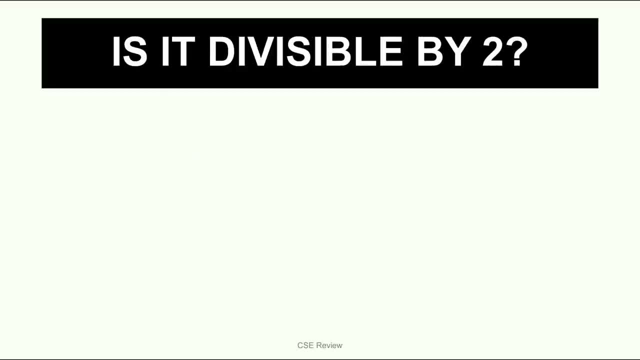 master them, so we'll discuss them one by one. Alright, so the first one that we discussed is if it is divisible by two. Now, this is actually fairly easy because it's something that we discussed earlier in childhood, but we'll establish it because, again, you have to master the entire thing. So what? 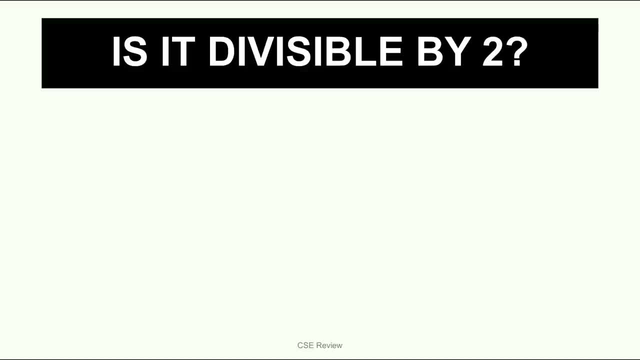 we're going to talk about today. in order for you to know how to master it is that you have to practice. if a number is divisible by two, you have to determine the rule. Ang rule for divisible by two na numbers is: if it is even So, if you're not familiar with your numbers, meron tayong odd. 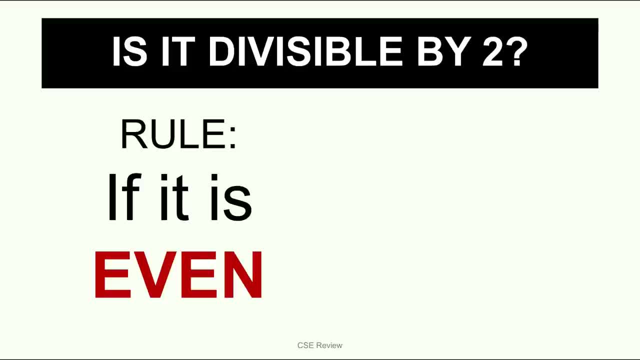 numbers. meron tayong even numbers. If a number is odd, then it is not divisible by two. If it is even, then it is divisible by two. Now, how do you know that A number is even if yung kanyang ending? 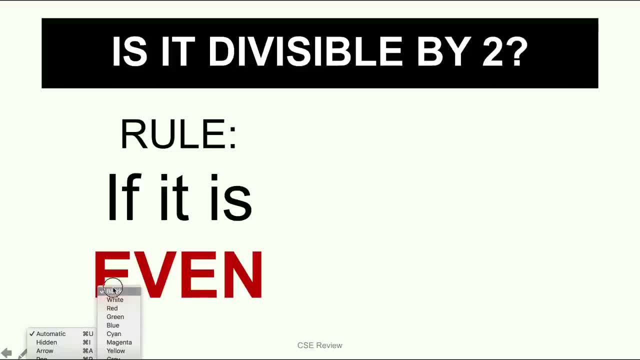 na number is also an even number. Ano ibig sabihin doon? If ang ending or ang dulong digit is zero, two, four, six and eight, then it is. even If hindi siya yung mga numbers na yan, then it is. 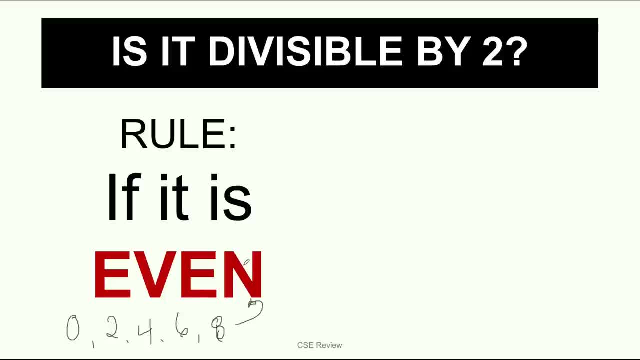 not divisible by two, and it is not even Now. here's what we're going to do today. I'm going to give you a list of numbers right here on the side, and then we're going to determine if they are divisible by the number that we're talking about. Okay, together. 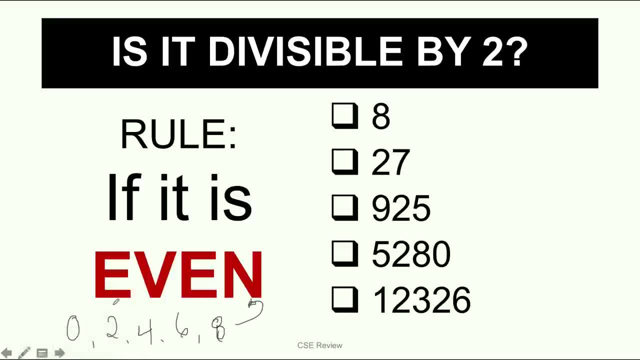 So ang gagawin natin, iisa-isayin natin ito to figure out kung divisible ba siya sa two. Now, this number here, number eight, it is not divisible by, it is divisible by two, kasi eight yung ending na. 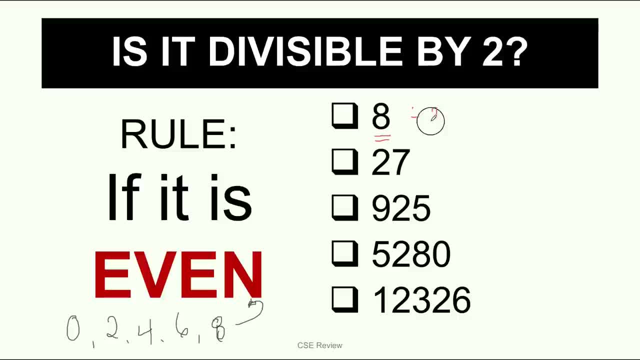 number or dulong digit niya. And if you check it, eight divided by two is four. Ang ibig sabihin lang ng divisible is whole number. dapat yung magiging sagot: Eight divided by two is four. So ibig sabihin: 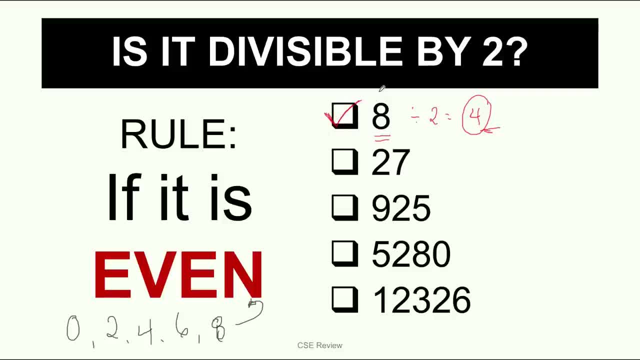 it is divisible by two. So check tayo dyan. Okay, Now twenty-seven, Ano, ang dulong number niya. Ang dulong number niya ay seven, and seven is not divisible by two, kasi seven divided by two is. 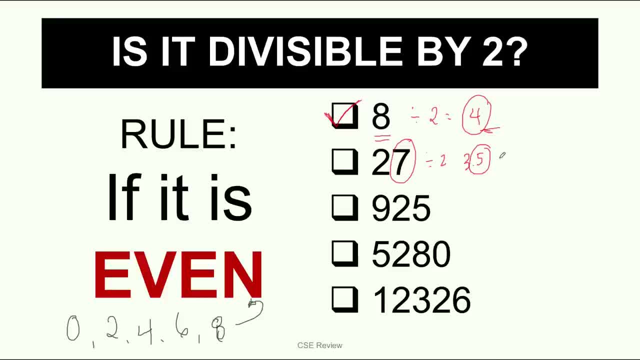 I'm going to give you three. point five, Again point five. Ibig sabihin, nun may butal. and again, this is an odd number. so hindi siya, even hindi siya, divisible by two. Okay, I want you to get. 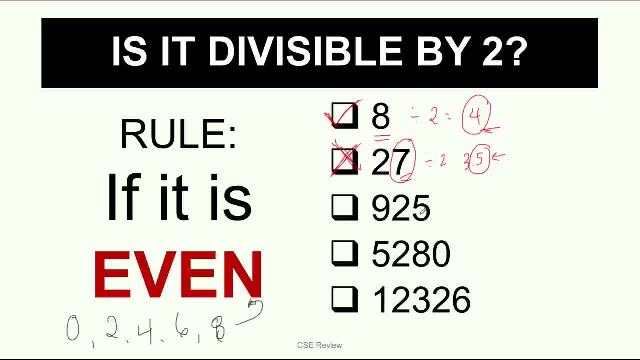 the hang of it Now, nine hundred and twenty-five naman tayo. Nine hundred and twenty-five dulong number is five. Five divided by two, hindi pwede. This is going to give you two point five Decimal din yan, hindi din pwede. 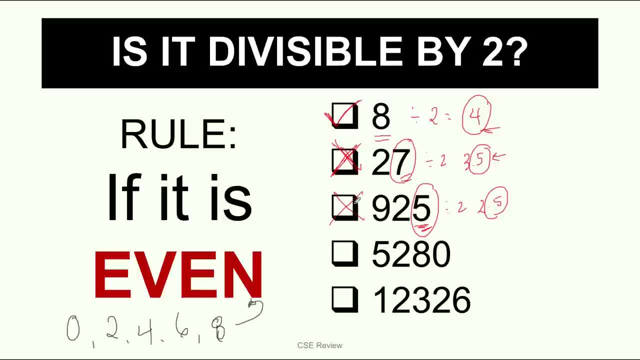 And again odd number siya, So x Again. the more you do it, the faster you get, So zero again. pasok siya dun, so pwede siya Six. pasok siya, so pwede siya sa two. Anong ibig sabihin nun? 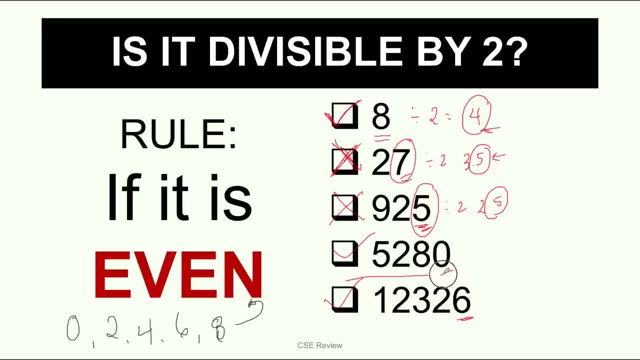 If you are reducing a fraction into lowest terms. for example, you have five to eighty Kunyari lang ha, five thousand two hundred eighty over one, two, three, two, six, To reduce it to lowest terms, two. You can start with that And then go and go and go Alright. So that is sa two. 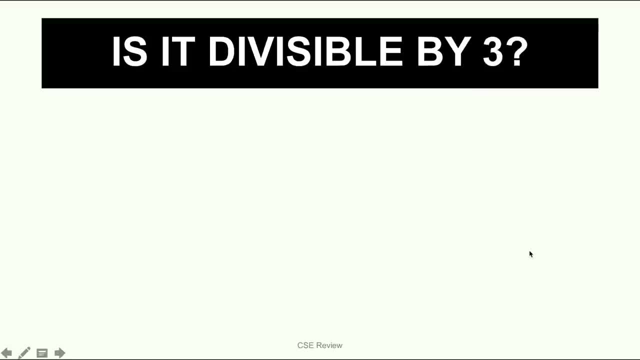 Lilipat naman tayo sa three. Now this is a little bit trickier, but I know you can figure it out. A number is divisible by three. Ito ang rule. The rule is if the sum of its digits is divisible by three. 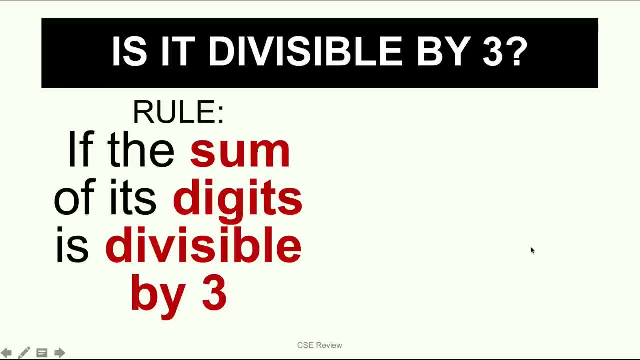 Now a few things I need to point out. If the sum of its digits ano, ibig sabihin nun Bawat isang digit, iya-add mo siya together to get it, And then yung mismong sum. 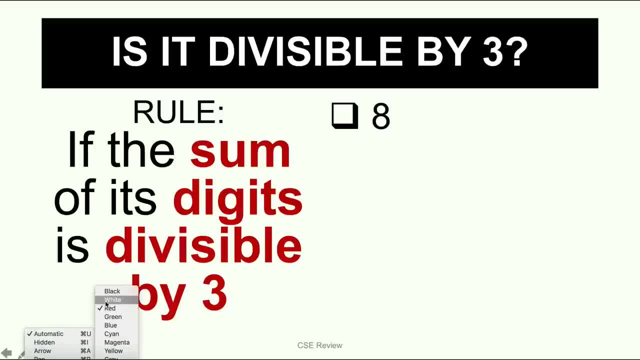 pinagdugtong-dugtong. yun ang magiging rule dun babase: if it's divisible by three, So ano yung digits niya. And if it is divisible by three, So eight. okay, Divided by three hindi pwede. 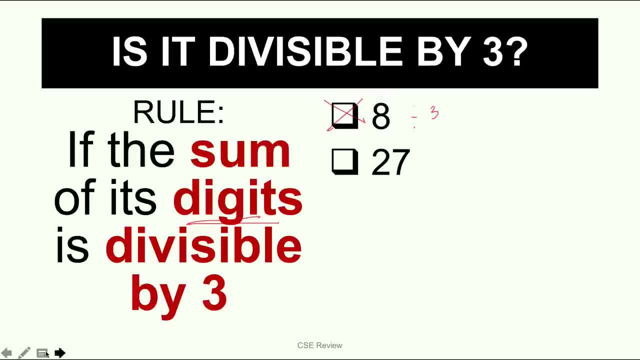 Okay, So this is not divisible by three. Next number tayo two and seven or twenty-seven. So ang gagawin lang natin is we're going to add two and seven, So two plus five. eh, two plus seven is. 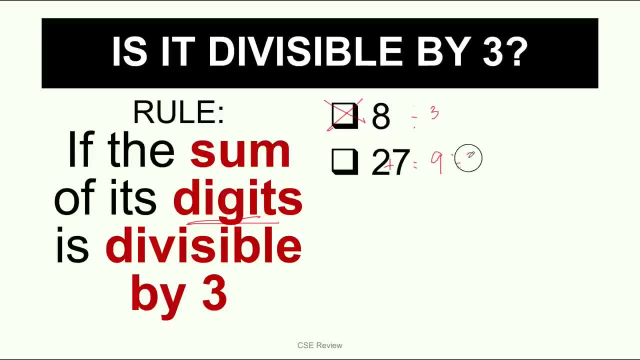 nine and then nine divided by three is pwede, kasi nine divided by three is going to give you three, okay, Then this is divisible by three. Two plus seven. Iya-add mo lahat ng digits. Next number tayo. okay. 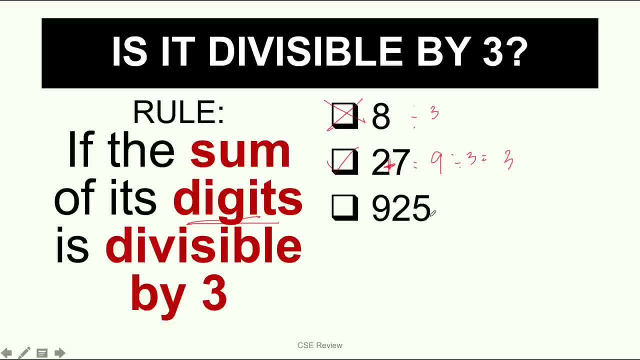 Yung. next number natin is nine to five. Again, it looks complicated. kung iya-try line, error mo siya. pero again ang gagawin lang natin, iya-add natin lahat ng digits. So nine plus two plus five is equal to nine plus two is eleven plus five is sixteen. 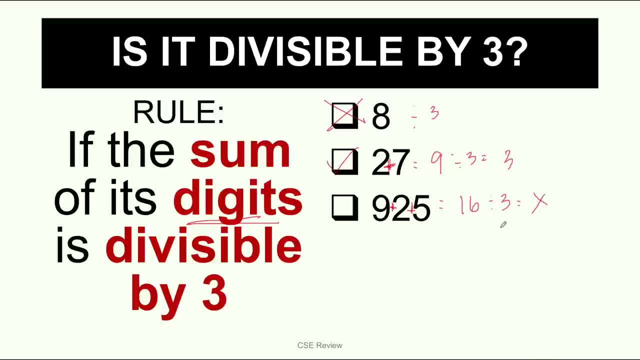 Now yung sixteen divided by three, hindi siya pwede. okay, Kasi fifteen pwede, pero sixteen hindi. may butal Pag may butal or may remainder or may decimal hindi. So this is not divisible by three, okay. 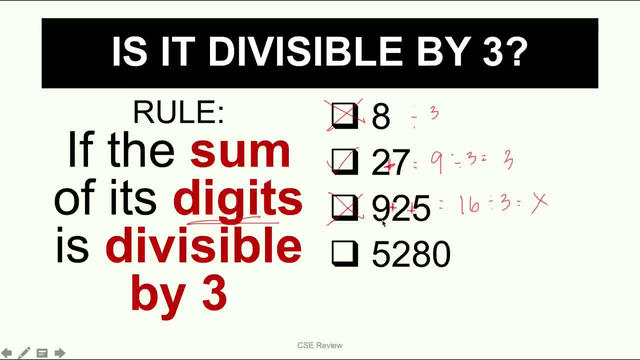 Now level up tayo Again. this is an even bigger number. You have five to eight zero. So anong gagawin natin? iya-add natin siya lahat: Five plus two plus eight plus zero. Five plus two is seven plus eight is going to give us fifteen. 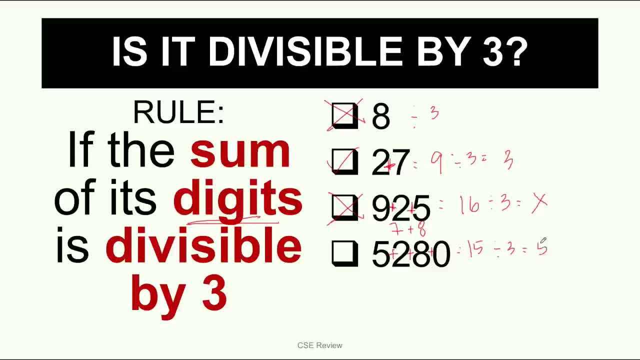 So anong gagawin natin? iya-add natin siya lahat: Five plus two plus eight plus zero. Five plus two is seven plus eight is going to give us fifteen. Fifteen divided by three, pwede na? Kasi that is five. So ibig sabihin, nun, this number is divisible by three. 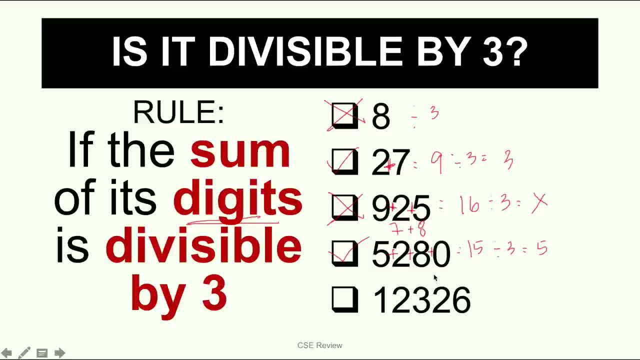 Next: one, two, three, two, six. Again looks complicated, Malaki, yung number, but it's really fast. Ang gagawin lang natin, iya-add natin siya lahat. So one plus two plus three, plus two plus six, So here you have three plus three, six. Dalawang six Twelve plus two is fourteen. okay. 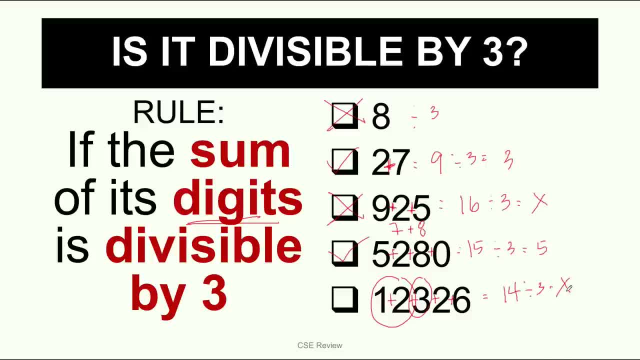 Fourteen divided by three is hindi pwede, kasi may butal. Okay, Anong gagawin natin? Ang gagawin na natin is hindi na kakross out na natin, to Hindi na siya divisible sa three. Okay, 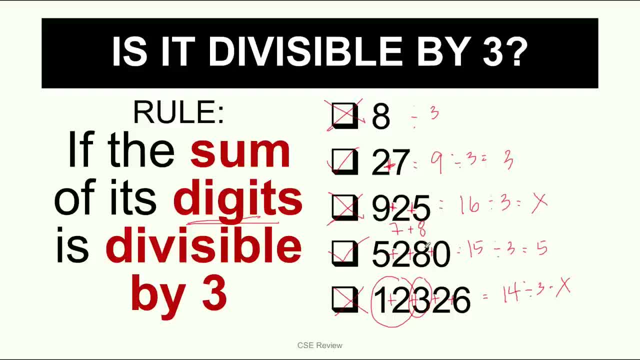 Bakit, Kasi, ang magiging divisible lang sa three ay any number na may sum ng digits na divisible by three rin. Okay. So again, anong kailangan tandaan? The sum of the digits has to be divisible by three. 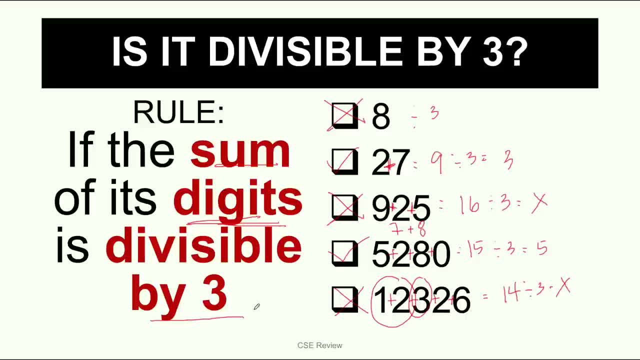 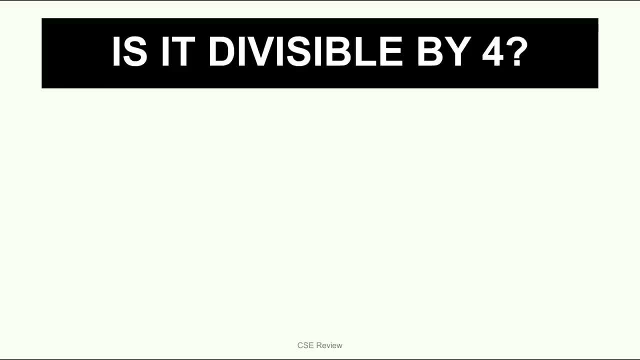 3.. Now you know how to deal with the number 3. Taas tayo ng level onte, puto tayo sa 4.. Again, may rule siya. A common mistake is most people think na basta even number pwede sa 4.. 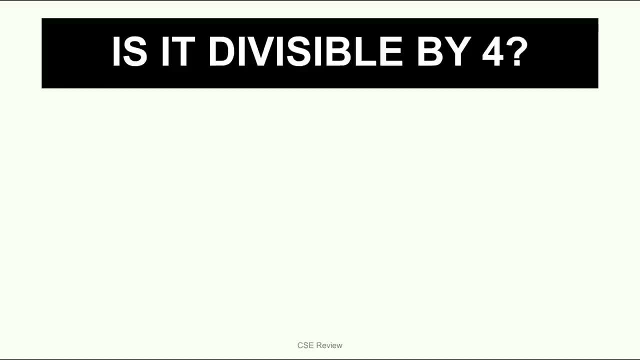 And that's not true. okay, There are even numbers na hindi pwede sa 4.. For example, 6.. 6 divided by 4 is 1 and a half, So hindi siya pwede, kasi meron siyang butal. 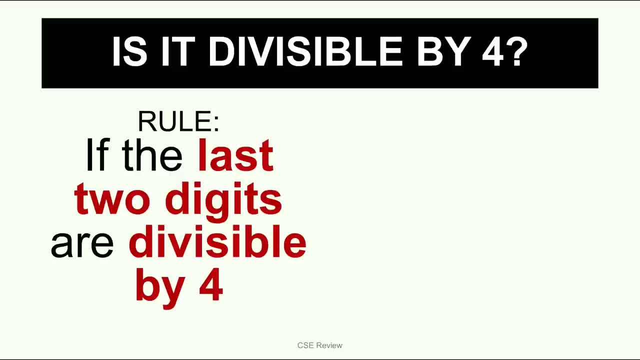 So ano ang rule? Ang rule is if the last 2 digits are divisible by 4.. Again, anong titignan natin Yung last 2 digits? Ngayon? paano kung isang digit lang siya like 8?? 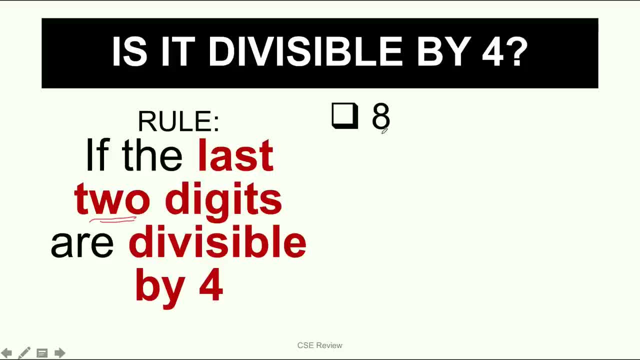 Okay lang yan, no problem, Kasi kung ano lang yung digit na meron, So 8 divided by 4, pwede ba 2. So it's really basic. pwede Taas tayo ng level 27.. 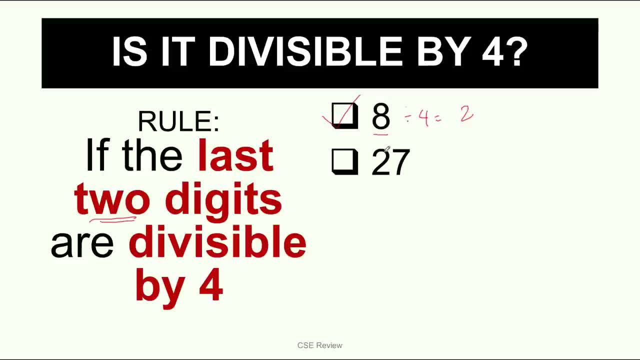 Again, anong gagawin natin? Look at the last 2 digits. So in this case it's not that helpful pa, So di-divide mo siya sa 4.. Meron kang butal, kasi you'd know na 24 ang 6,, 28 ang next. 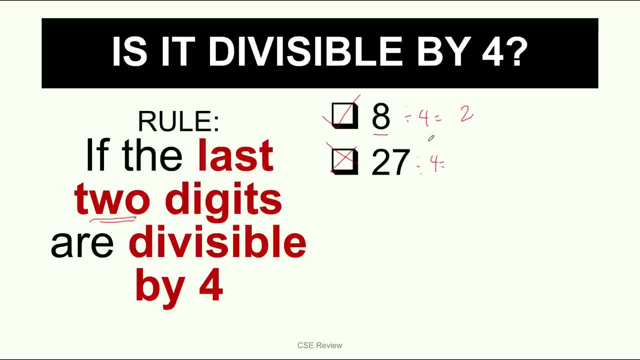 So kulang siya. So this is not divisible by 4.. Okay, Hindi siya pwede may butal kasi may decimal. Ngayon taas tayo ng level ulit. This is going to be helpful pag alam niyo yung technique at ganito yung number 3 digits mas madali. 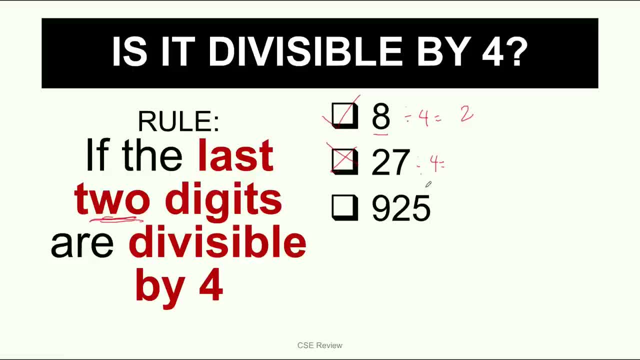 Okay, Bakit Kasi you're going to look at the last 2 digits? Ano, yung last 2 digits niya 25.. So kalimutan niyo muna yung 9.. Is 25 divisible by 4?? 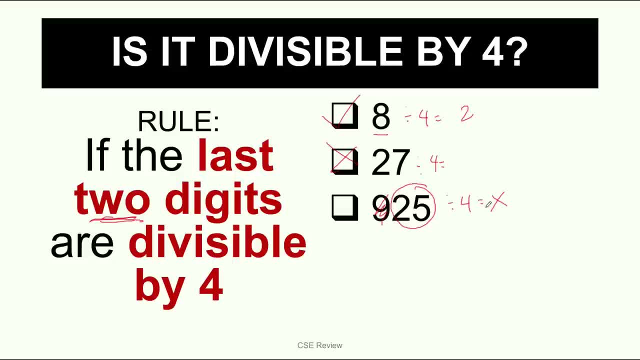 Hindi, Kasi 24.. Pwede, Pero 25, hindi. So anong gagawin nun? Ibig sabihin nun, ang 9, 25 is not divisible by 4.. Next, 5,, 2,, 8, 0.. 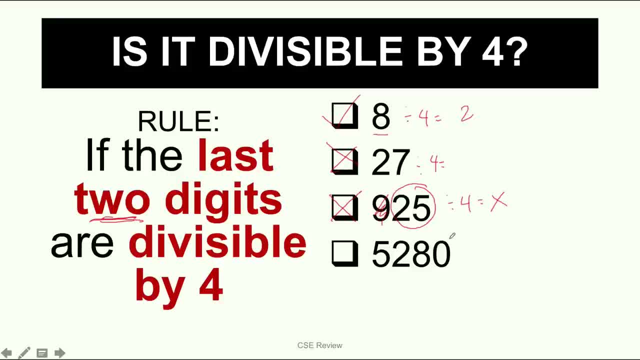 Again, ano ang rule natin, We are looking for the last 2 digits. Ano, yung last 2 digits niya 80. So is 80 divisible by 4? Pwede ba siya sa 4?? 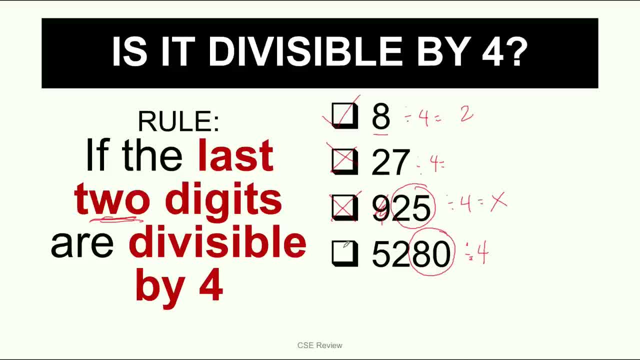 Yes, Kasi nga 80 divided by 4,, that's basically 20.. So ito pwede siya. Next number, even bigger number Again, don't be afraid, Kahit gano'n siya kalaki, ang titinan mo lang are the last 2 digits. 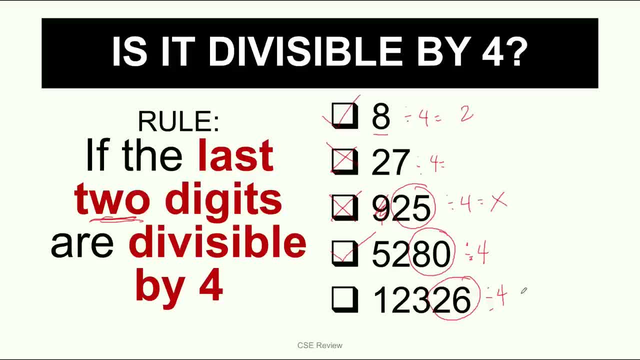 You have 26.. So is 26 divisible by 4?? No, Kasi kulang 24 pwede, pero 26 hindi. 28 pwede, 26 hindi. So ibig sabihin, nun, ito ay hindi divisible by 4.. 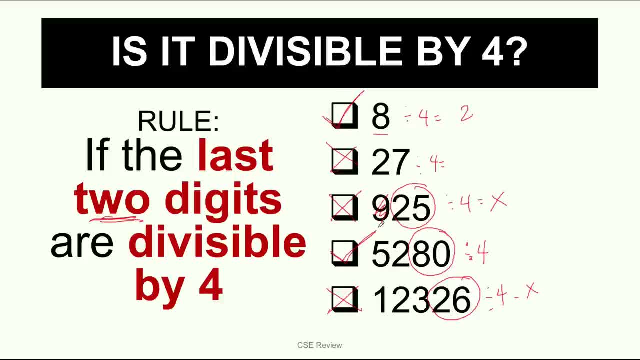 So ang divisible lang by 4 are 8 and 5, 2,, 8, 0.. Okay, So again, this is all about speed. The faster you are here, mas mabilis ka mag-radical, mas mabilis ka mag-factor 3,. 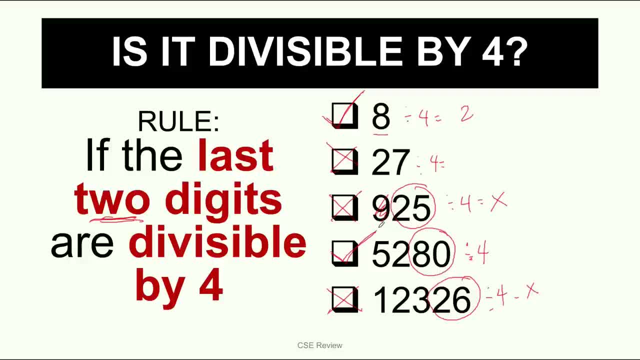 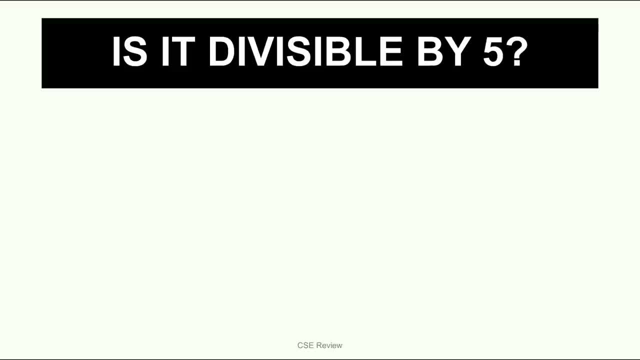 mas mabilis ka ngayon mag-solve Kahit polynomials. it's very important for you to know this. So is it divisible by 5?? This is actually the easiest technique of the bunch In order to know if a number is divisible by 5, the rule is this: 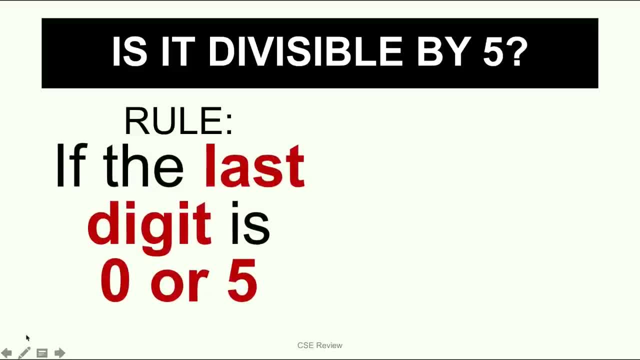 It has to have the last digit ng 0 or 5.. Again, 0 or 5 lang. So kung hindi 0 or 5, then automatic hindi siya divisible by 5.. So isa-isayin natin ngayon yung ating mga numbers here. 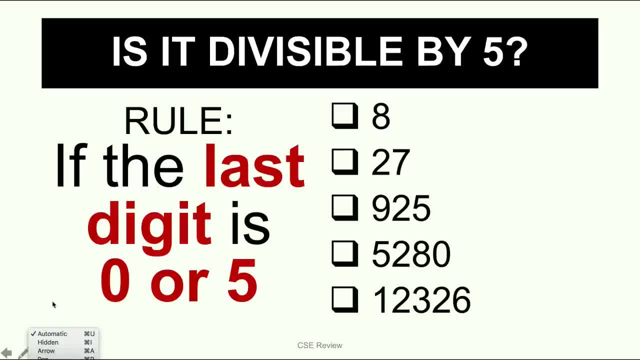 You have 8.. Ang 8 is not divisible by 5, kasi ang 8 is not 0 or 5, so hindi ito pwede 7, hindi rin siya pwede 5, pwede siya. 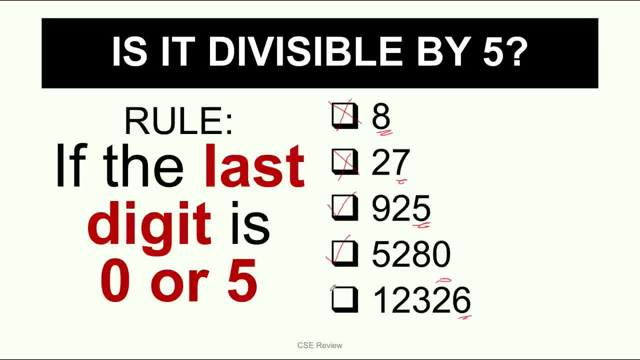 0, pwede siya And itong 6, hindi pwede. So x Now paano ito nakakatulong? If again, if you have a fraction na 5,, 2,, 8,, 0 over 1,, 2,, 3,, 2,, 6,.